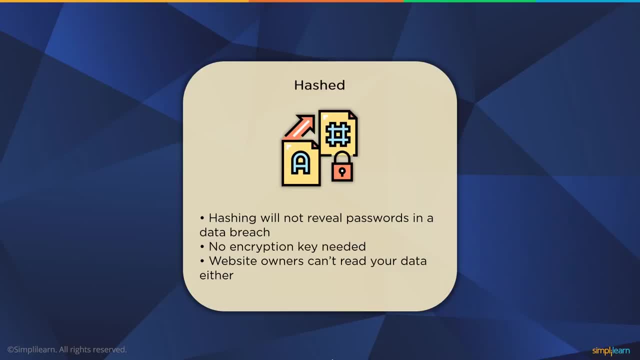 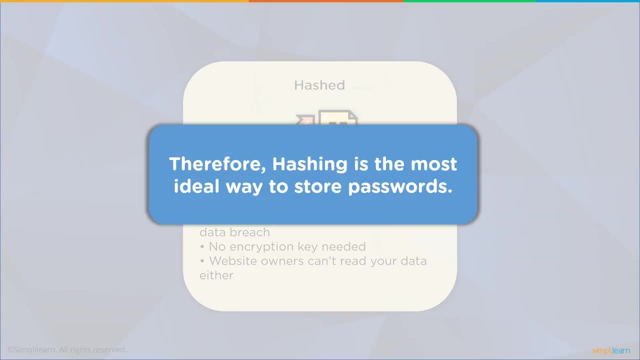 passwords to protect your credentials are safe from the website administrators. Considering all the pros, hashed passwords are the industry standard when it comes to storing credentials nowadays. Hey everyone, this is Bhavru from Simply Learn. Welcome to this video on what is hashing. 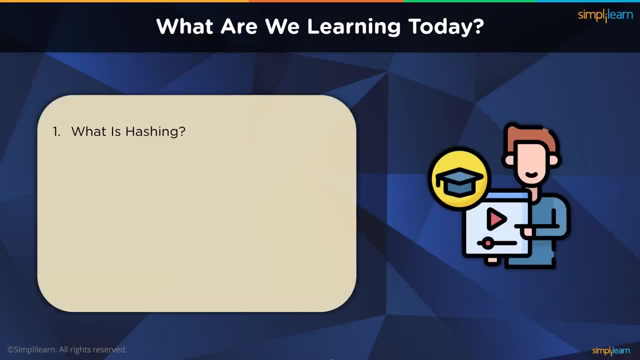 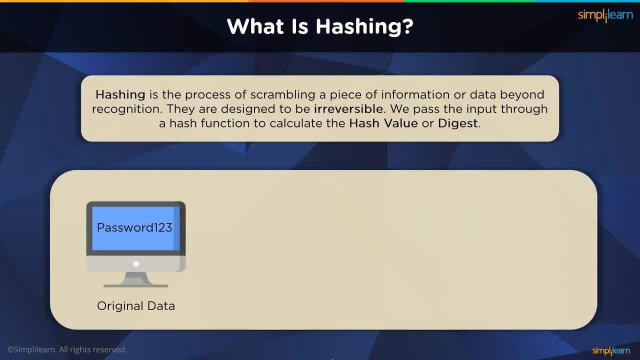 to hash functions. We move on to hash functions. We move on to hash functions. We move on by using hash functions, which are essentially algorithms that perform mathematical operations on the main plaintext. The value generated after passing the plaintext information through the hash function is called the hash value digest or, in general, just the hash of the original data. 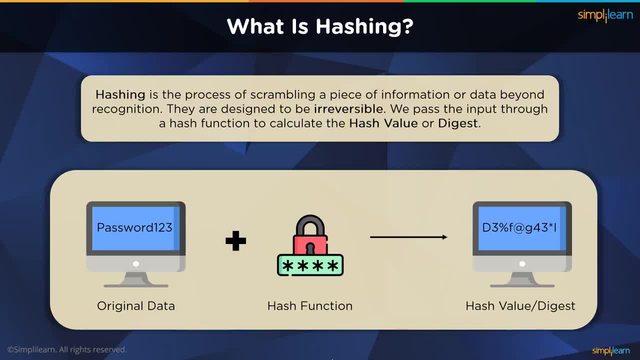 While this may sound similar to encryption, the major difference is hashes are made to be irreversible. No decryption key can convert a digest back to its original value. However, a few hashing algorithms have been broken due to the increase in computational complexity of today's new generation computers and processors. There are new algorithms that stand the test of. 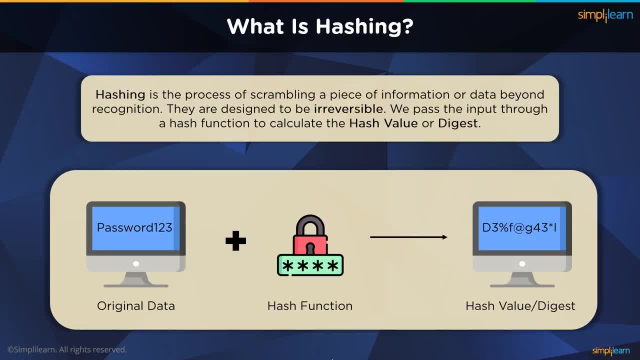 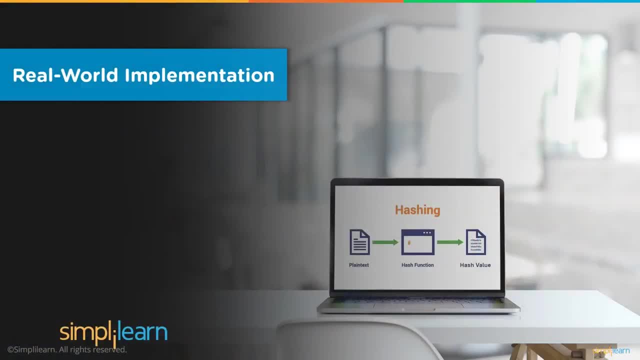 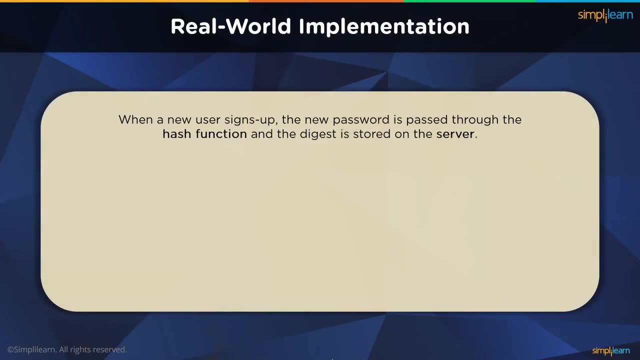 time and are still in use among multiple areas for password storage, identity verification, etc. Like we discussed earlier, websites use hashing to store the user's passwords. So how do they make use of these hash passwords When a user signs up to create a new account? 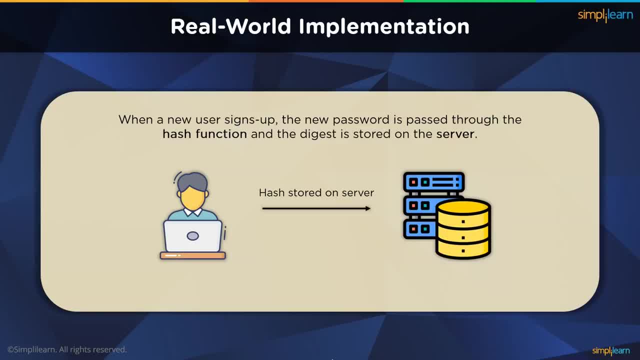 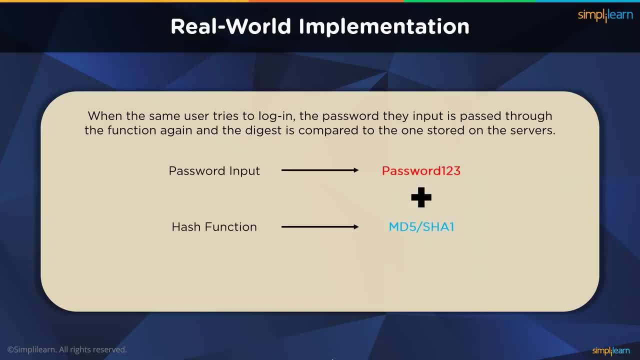 the password is there to be used. The user can run through the hash function and the resulting hash value is stored on the servers. So the next time a user comes to log into the account, the password he enters is passed through the same hash function and compared to the hash stored on the main server. 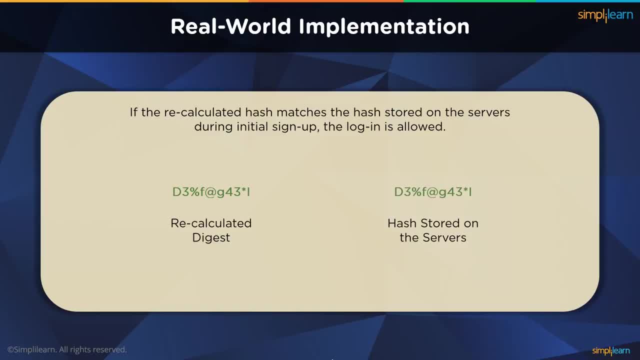 If the newly calculated hash is the same as the one stored on the website server, the password must have been correct because, according to hash functions terminology, same inputs will always provide the same outputs. If the hashes do not match, then the password must be correct. If the hashes do not match, then the password must be correct. 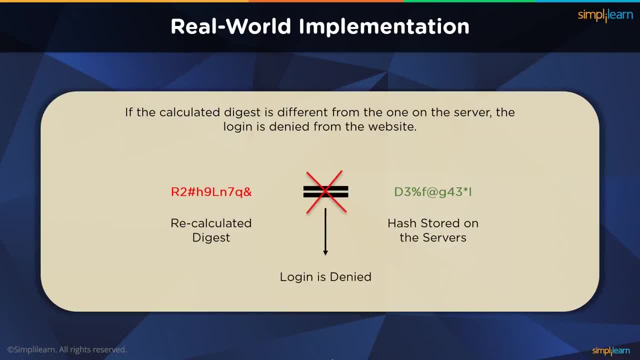 The password entered during login is not the same as the password entered during the signup. hence the login will be denied. This way, no plaintext passwords get stored, preventing both the owner from snooping on user data and protecting users' privacy in the unfortunate event of a data. 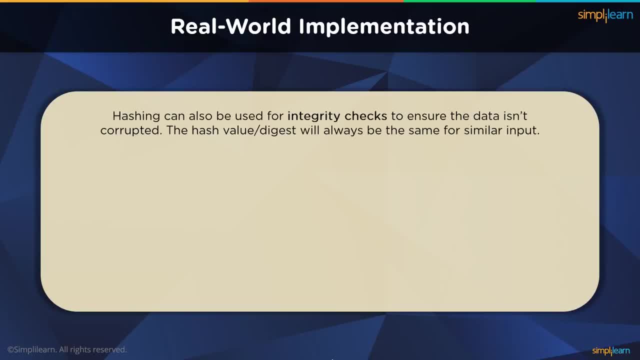 breach or a hack. Apart from password storage, hashing can also be used to perform integrity checks. When a file is uploaded on the internet, the file's hash value is generated and it is uploaded along with the original information. When a new user downloads the file, he can. 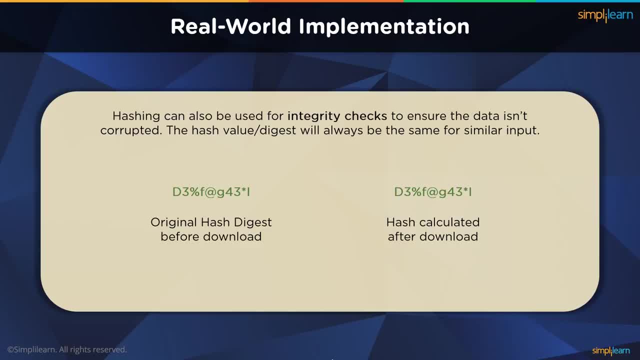 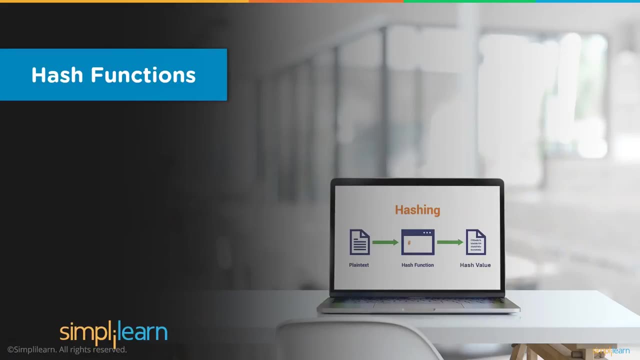 calculate the digest of the downloaded file using the same hash function. When the hash values are compared, if they match, then file integrity has been maintained and there has been no data corruption, Since so much important information is being passed onto the hash function. 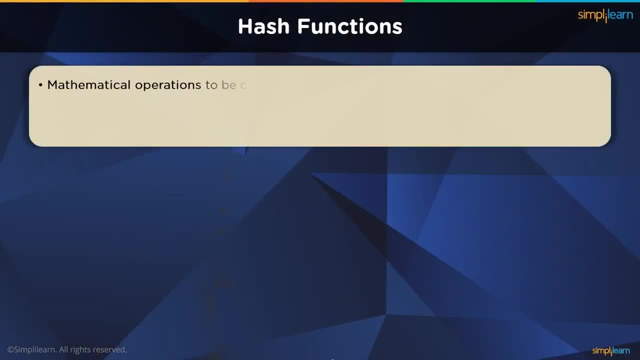 we need to understand how they work. A hash function is a set of mathematical calculations operated on two blocks of data. The main input is broken down into two blocks of similar size. The block size is dependent on the algorithm that is being used. Hash functions are designed to be one-way. They shouldn't be reversible, at least by design. 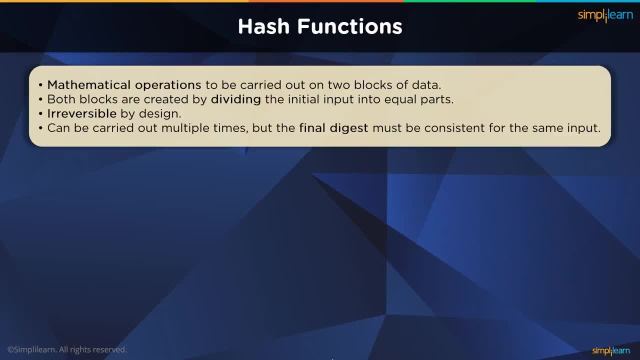 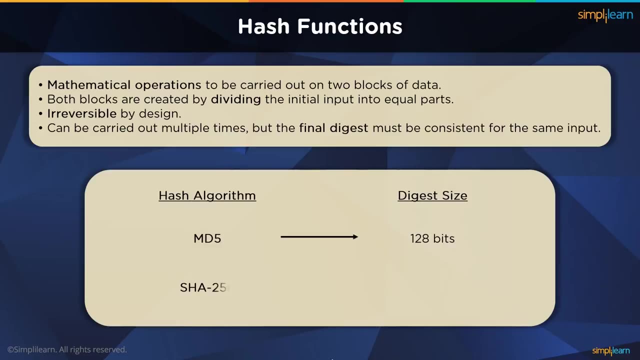 Some algorithms, like the previously mentioned MD5, have been compromised, but more secure algorithms are being used today, like the SHA family of algorithms. The digest size is also dependent on the respective algorithm being used. MD5 has a digest of 128 bits, while SHA256 has a digest of 256 bits. 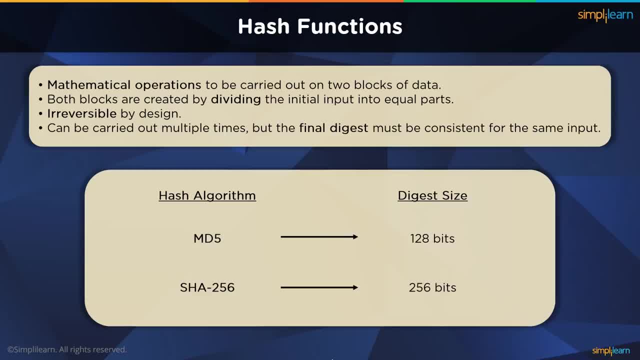 This digest must always be the same for the same input, irrespective of how many times the calculations are carried out. This is a very crucial feature, since comparing the hash value is the only way to check if the data is untouched, as the functions are not reversible. 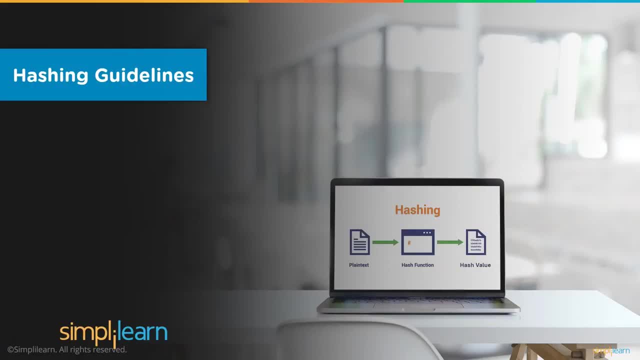 There are certain requirements of a hash function that need to be met before they are accepted. While some of them are easy to guess, others are placed in order to preserve security in the long run. The hash function must be quick enough to encrypt large amounts of data at a relatively fast pace. 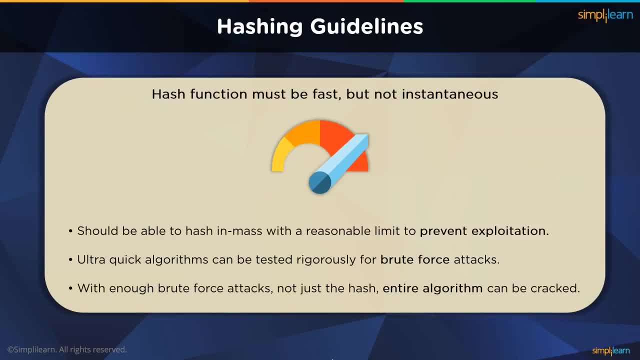 but it also shouldn't be very fast. Running the algorithm on all cylinders makes the function easy to bootforce and a security liability. There must be a balance to allow the hash function to handle large amounts of data and not make it ridiculously easy to bootforce by running through all possibilities. You need to be open to the need to handle large amounts of data and not make it ridiculously easy to bootforce by running through all the possibilities. 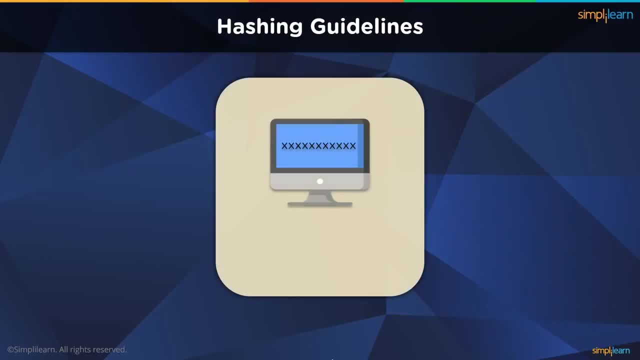 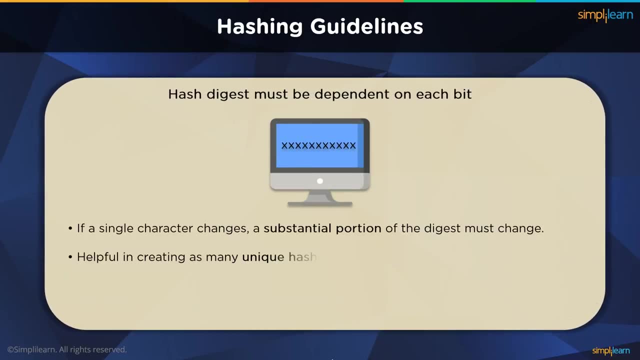 combinations. The hash function must be dependent on each bit of the input. The input can be text, audio, video or any other file extension. If a single character is being changed, it doesn't matter how small that character may be. the entire digest must have a distinctly different hash value. This is essential. 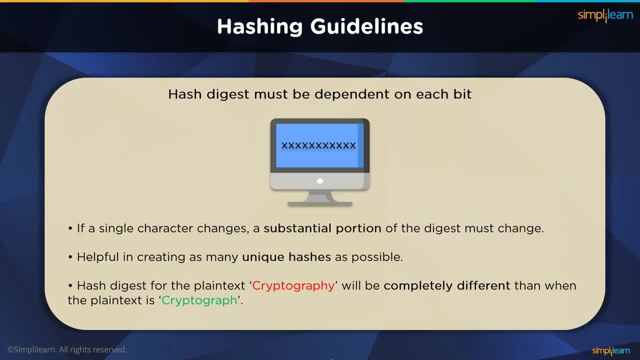 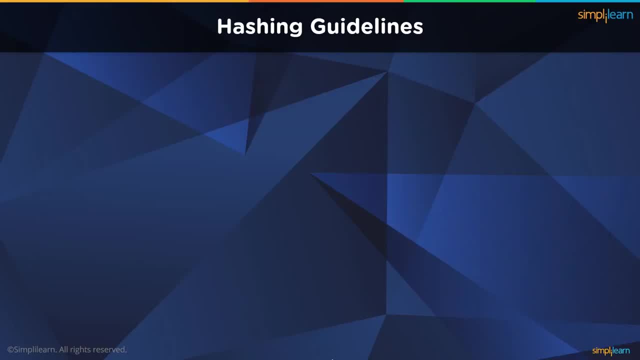 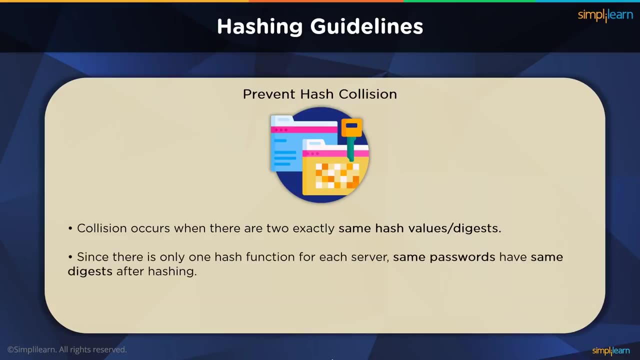 to create unique digests for every password that is being stored. But what if two different users are using the same password? Since the hash function is the same for all users, both the digests will be the same. This is called a hash collision. You may think this must be a rare occasion where two users have 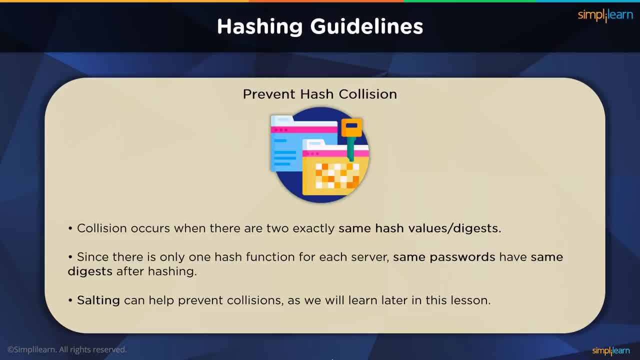 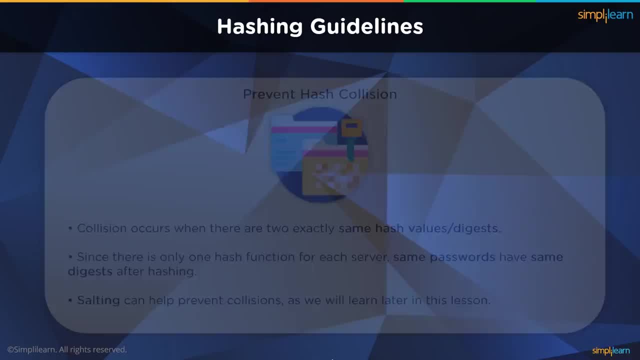 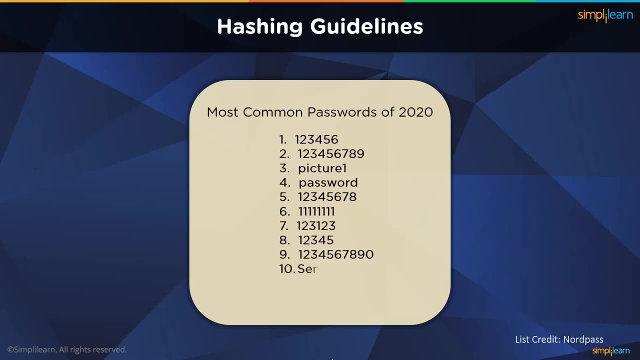 exactly the same password, but that is not the case. We have techniques like salting that can be used to reduce these hash collisions, as we will discuss later in this video. You would be shocked to see the most used passwords of 2020.. All of these passwords are laughably insecure and since many people use the 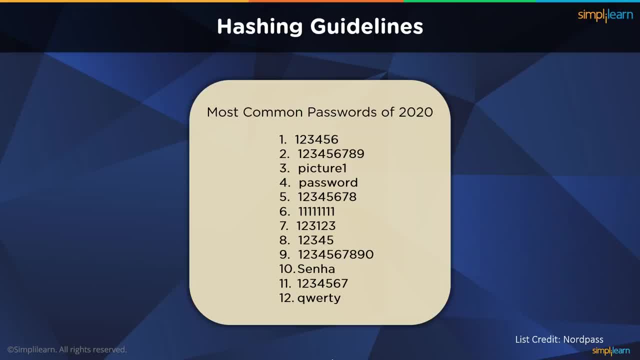 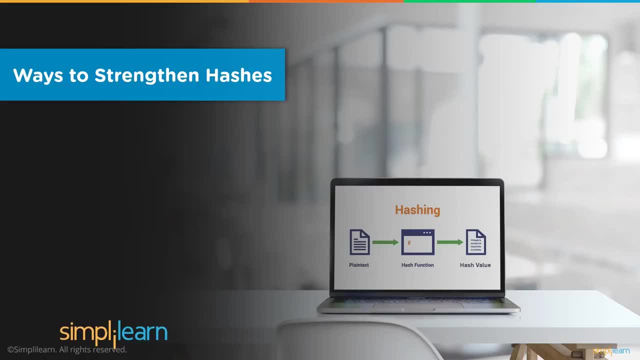 same passwords repeatedly on different websites. hash collisions are more common than one would expect. Let's say the hash functions find two users having the same password. How can they store both the hashes without messing up the original data? This is where salting and peppering come to play. 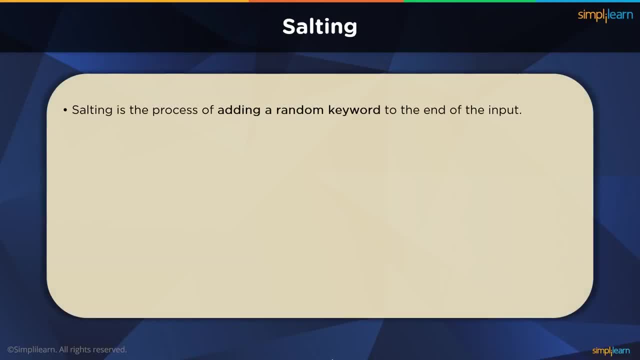 Salting is the process of adding a random keyword to the end of the input before it is passed on to the hash function. This random keyword is unique for each user on the system and it is called the salt value or just the salt. So even if two passwords are exactly the same, the 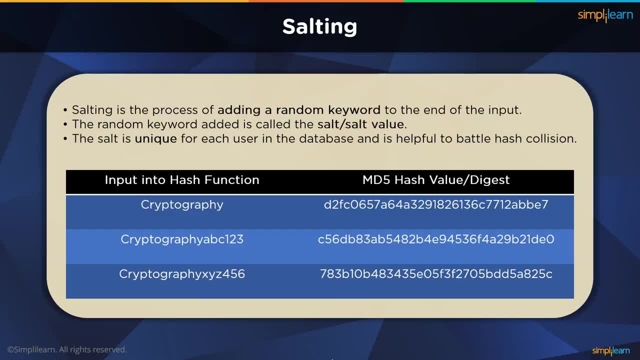 salt value will differ, and so will their digest. There is a small problem with this process, though. Since the salt is unique for each user, they need to be stored in the database along with the passwords and sometimes even in plain text, to speed up the process of continuous verification. If the server is 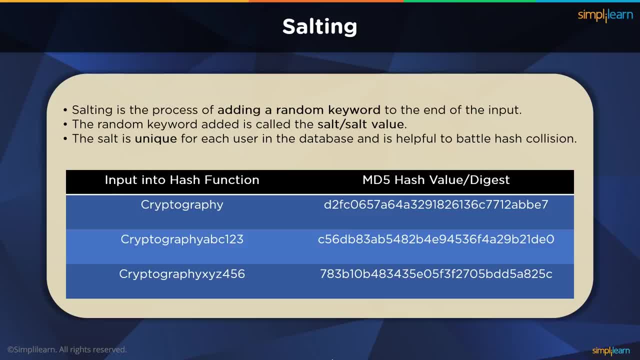 hacked, then the hashes will need to be forced, which takes a lot of time, But if they receive the salts as well, the entire process becomes very fast. This is something that peppering aims to solve. Peppering is the process of adding a random string of data to the input. 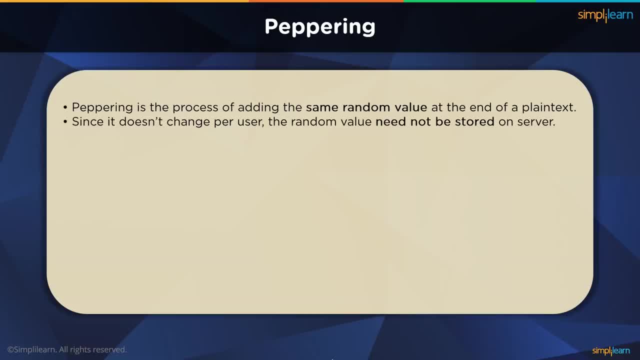 before passing them to the hash function. But this time the random string is not unique for each user- It is supposed to be common for all users in the database- and the extra bit added is called the pepper. in this case, The pepper isn't stored on the servers. 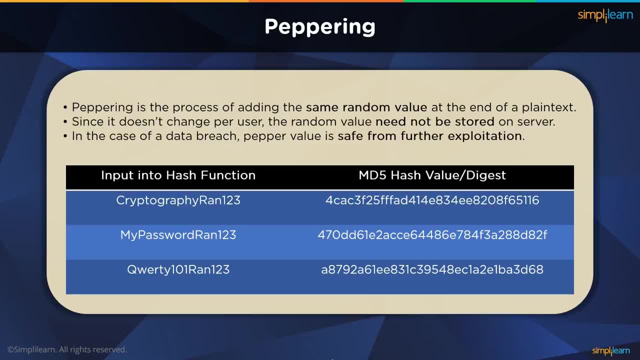 It is mostly hard coded onto the web's source code, since it's going to be the same for all credentials. This way, even if the server gets hacked, they will not have the right pepper needed to crack into all the passwords. Many websites use a combination of salting and peppering to solve the 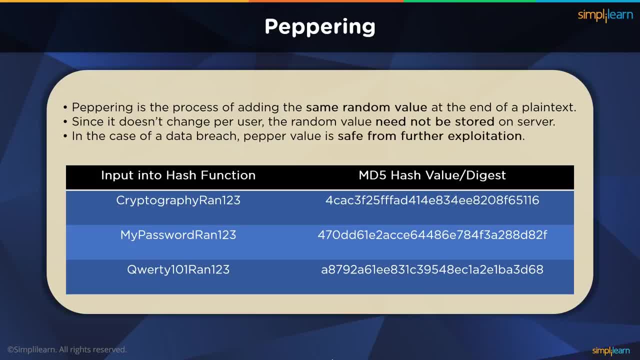 problem of hash collusion and bolster security. Since brute force takes such a long time, many hackers avoid taking the effort. The returns are mostly not worth it and the possible combinations of using both salt and pepper makes this so hard to hack. netting and peppering is humongous.